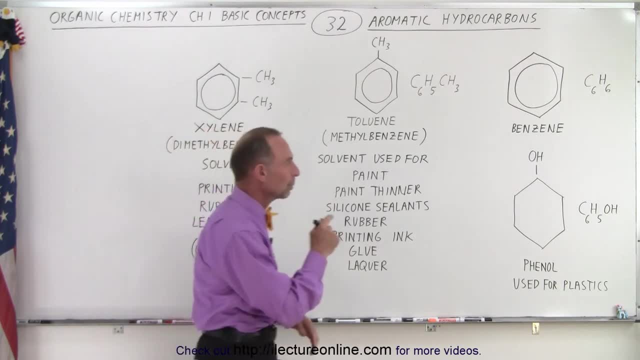 particular molecule. Now notice that when we replace one of the two, we have a different hydrogen. So when we replace one of the hydrogens with an OH, it becomes phenol, And that's the common name of that particular molecule. And of course I'm missing something here. We still have 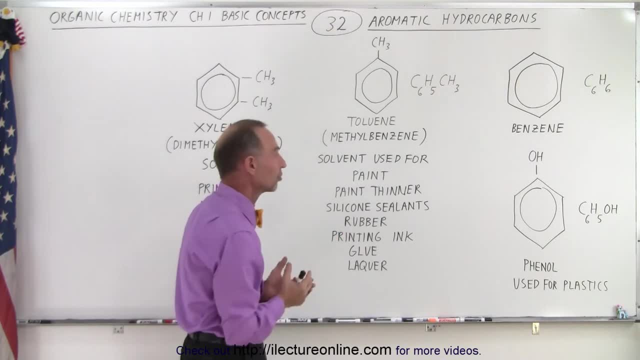 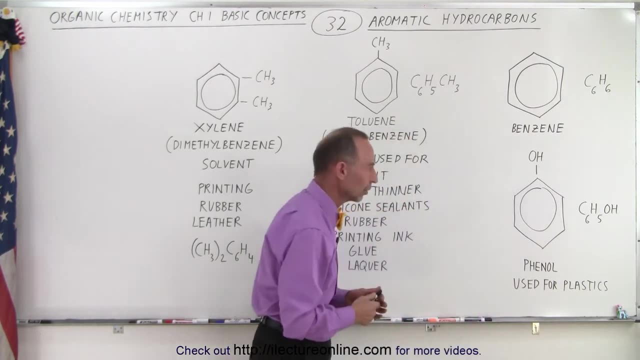 the ring symbol inside because it is a ring structure And so when we replace one of the hydrogens with an OH, then it becomes phenol, And that's something that we use for plastics And notice the chemical equation is written as C6H5 with an OH attached at the end. Then if we take 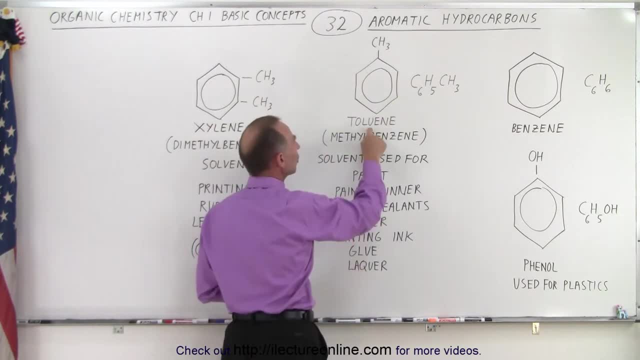 hydrogen and replace it with a metal group, then it's called toluene. So we have OH, it's called phenol. We have the metal group, we call a toluene. Of course the proper name would be methylbenzene. 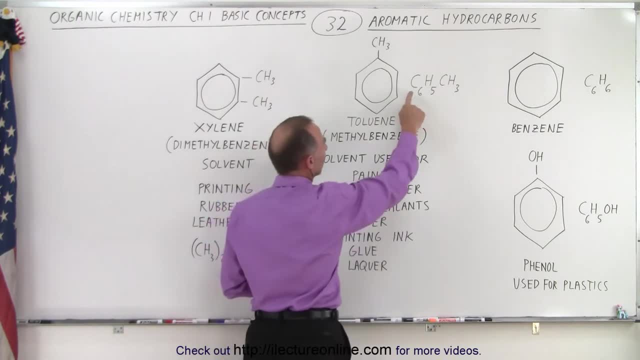 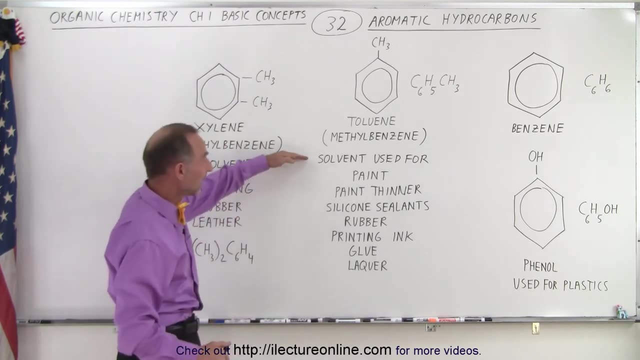 the metal addition to the benzene ring, And there we write C6H5CH3.. Now, this has a lot of different uses. Notice, it's a solvent and it's used for paint, paint, thinner, silicon, sealant, rubber, printing ink, glue, lacquer, you name it. It's a very 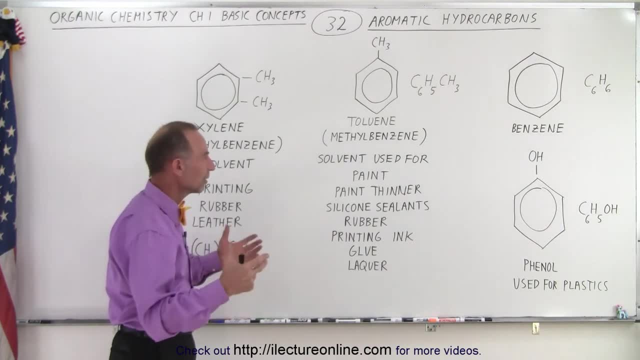 very ubiquitous molecule that we use in a lot of different industrial practices. So that's again where the paint thinner came from And that's of course I really liked that smell as a kid. Not good to sniff it, not good to smell. It's not very healthy to get those aromas into your lungs. 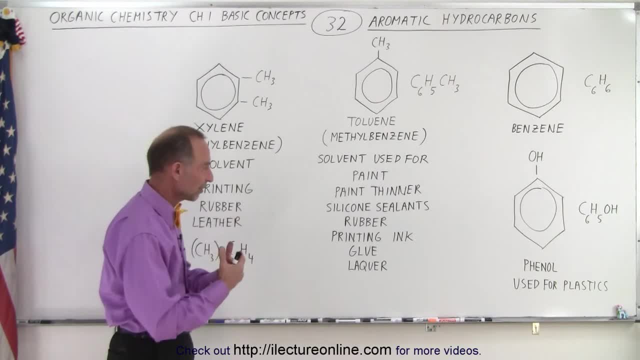 But yeah, that's why they're called aromatic hydrocarbons, because they have that very strong, very specific smell to them. And then if we, instead of having one metal group, we have two from toluene with a single metal group. Now we have two metal groups, we call it xylene, So instead 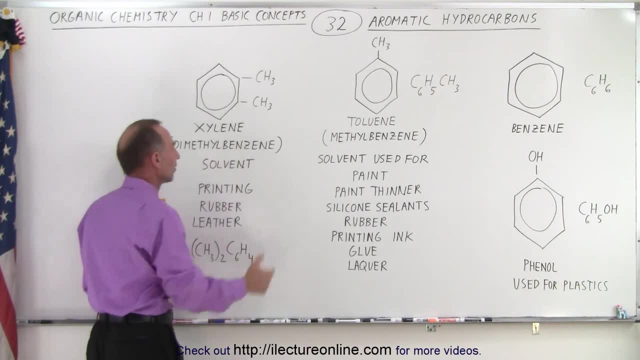 of calling it methylbenzene, since there's two of them, we call it dimethylbenzene. It's also a solvent and we use it for printing, for rubber and for the production of leather, to treat it in order to make it into a leather product. Notice: we have the CH3, there's two of them and that's. 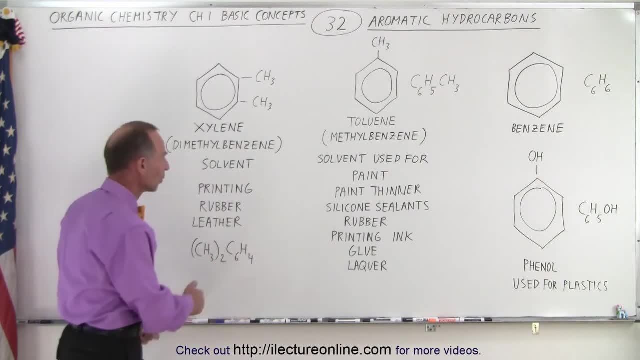 connected to a C6H4. So all of them have a C6, but notice that the more groups you attach instead of hydrogen, of course the number of hydrogens will decrease. So there's more hydrogen on this particular molecule. Notice that we write in such a way that